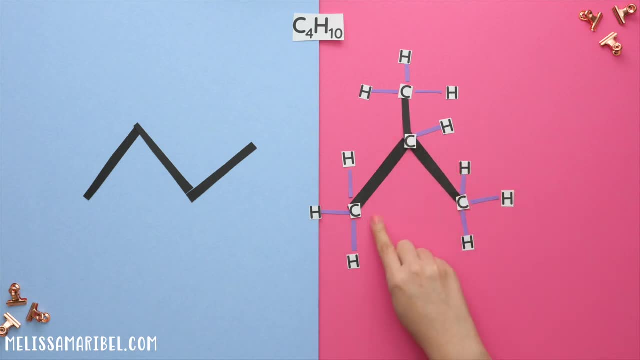 has three bonds, so it needs a hydrogen. here We have one, two, three, four carbons and one, two, three, four, five, six, seven, eight, nine, 10 hydrogens. If we were to move this methyl group here. 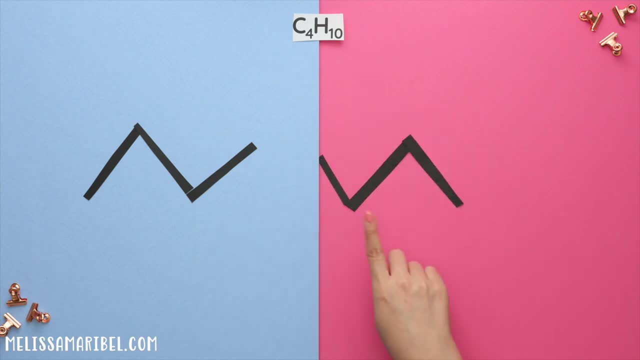 it wouldn't have been a constitutional isomer, because it is the same structure as the first one, just flipped around. So we only have two constitutional isomers. Sometimes we will be given a chemical formula that can have constitutional isomers that are either an alkane, an alkene or a cyclic ring. 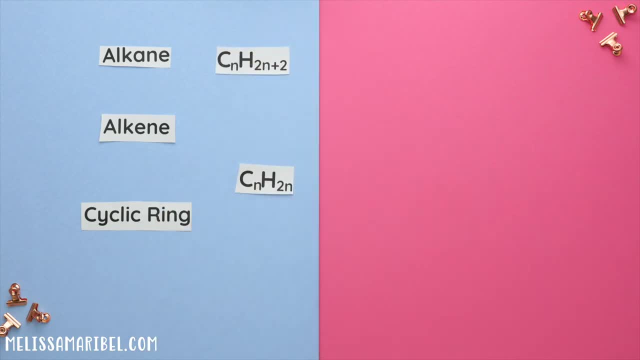 These two formulas will help you determine which type of structure you will draw. An alkane has this formula. In the previous example we had C4H10, where N is equal to four. We'll plug N into the formula of 2N plus two. 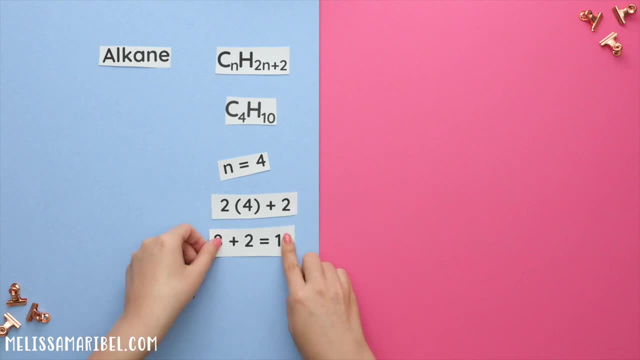 So multiply two times four to get eight plus two is 10.. So this is how we knew it was an alkyl. This is an alkane, meaning everything had a single bond For an alkene or cyclic ring. this is our formula. 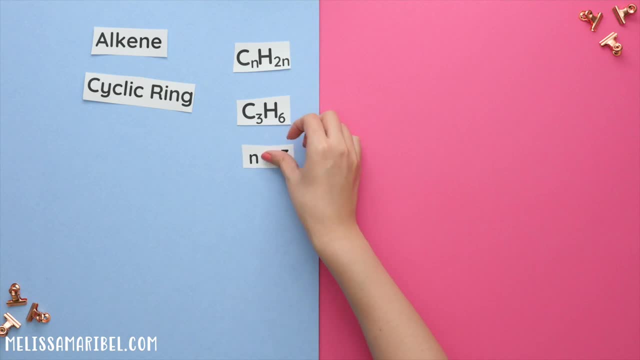 Let's say we had C3H6, where N is equal to three, And we will plug this into the formula of 2N to get two times three, which is six. So since it fits with the formula, the constitutional isomers can either be an alkene, 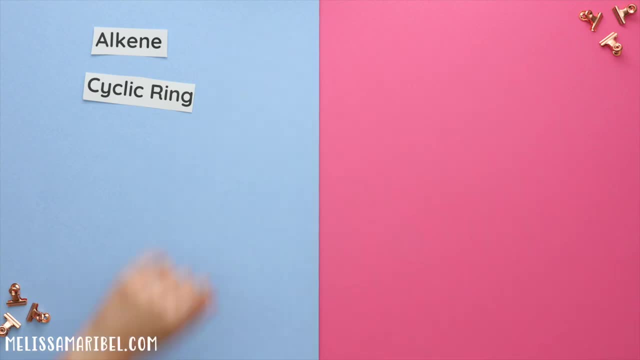 or a cyclic ring. Let's do two common test questions. The first one asks us to find all the constitutional isomers, and the second one asks us to find all the constitutional isomers for C6H14.. So start with identifying if this is an alkane. 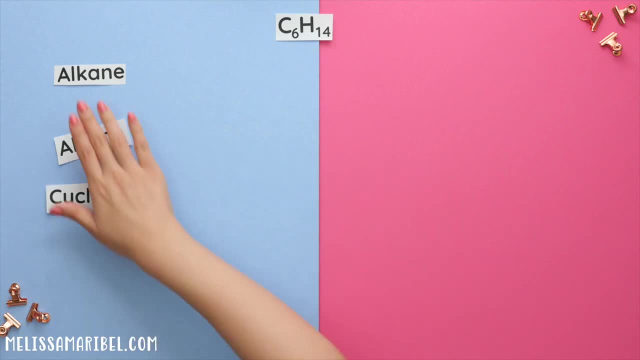 or an alkene or cyclic ring. We'll use the formula for an alkane first, where, in this case, N is six, Plug six into 2N plus two. Two times six is 12, plus two is 14.. So yes, this is an alkane. 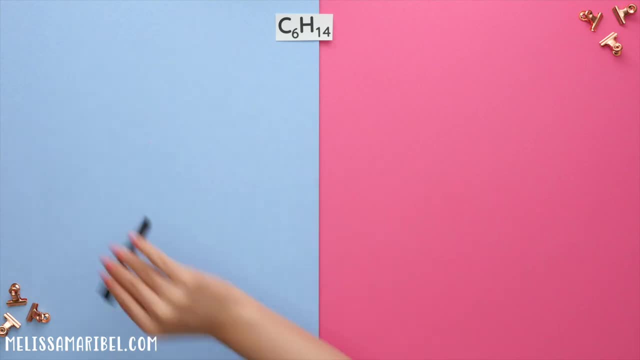 meaning everything will have a single bond. Now start with drawing the simplest structure. In our case it's the typical skeletal structure. Next, start moving a carbon chain to a different location and double-check that we still have the D same amount of carbons and hydrogens. 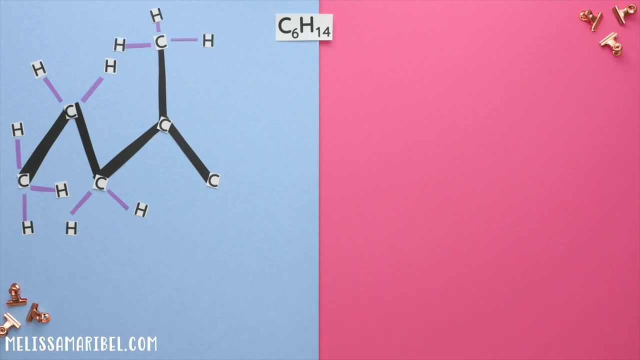 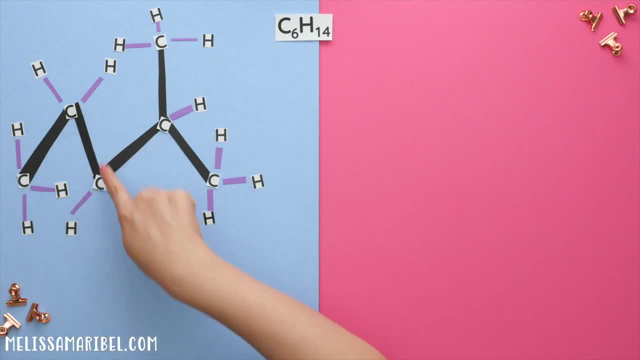 11,, 12, 13,, 11, 12, 13, 14 hydrogens and one, two, three, four, five, six carbons. Now let's move this carbon chain here and double-check our hydrogens. 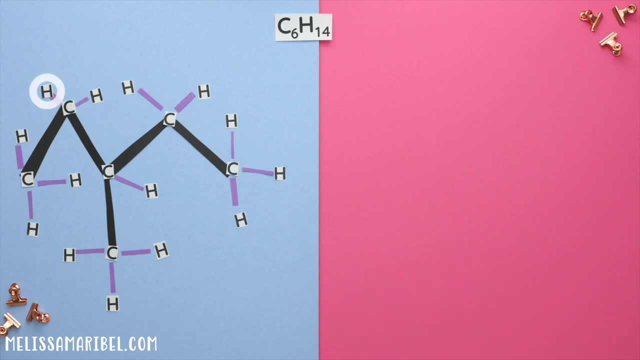 So three, six, nine, 10,, 11,, 12,, 13,, 14, and six carbons. We can keep going, so we'll move this carbon chain here, recount and yes, we have all 14 hydrogens and six carbons. 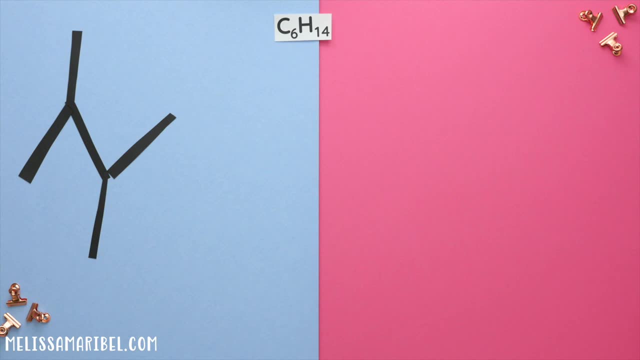 And next we'll move this carbon chain here and we again have 14 hydrogens and six carbons. If we were to move this back, it would revert to one of the isomers we already found. So that's how we know to stop. And we found all five constitutional isomers. The second question asks us to find all the constitutional isomers for C4H8.. So we'll check and see if this is an alkane or an alkene or cyclic ring. I'll start with the alkane formula where N is four. 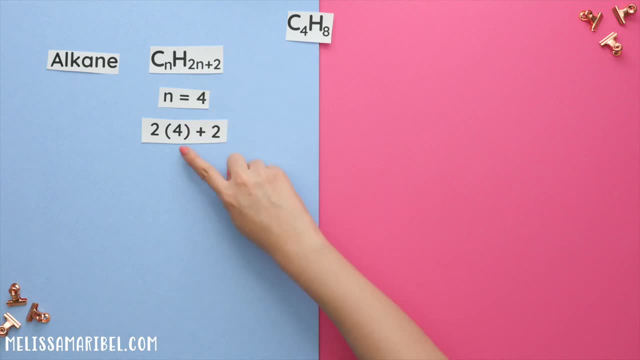 And if we were to plug in four for N, we have two times four is eight plus two is 10.. So no, it's not an alkane, since we have eight hydrogens and not 10.. I'll try the alkene slash cyclic ring formula. 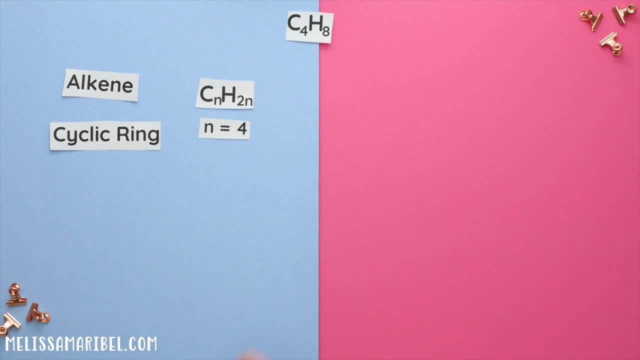 where N is four and we'll plug in four for N. so two times four is eight. So yes, this is an alkene and cyclic ring. Since we know it is an alkene, that is the first structure we will draw. 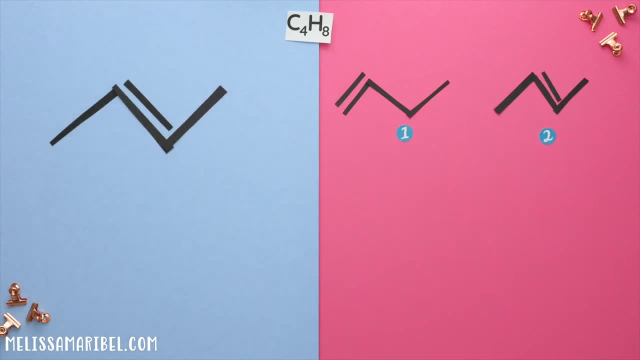 For the second isomer. we can move this double bond over. If we move it again to the N carbon, it is actually the same structure as the first original structure we just drew, But we can instead move this bond down. We now have a cis and trans isomer. 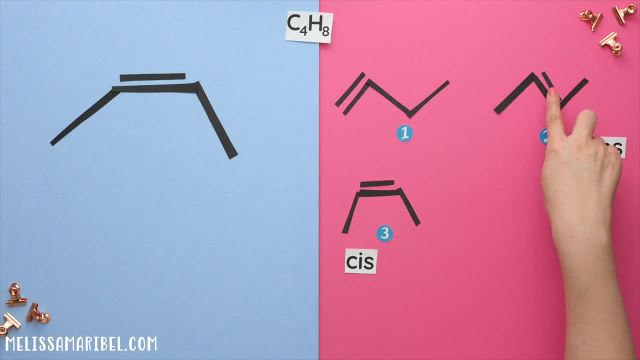 where trans refers to the substituents being on the opposite side of the double bond and cis refers to the substituents being on the same side of the double bond. Since there are no other ways to draw this alkane, we can now see if we can make this into a cyclic ring.